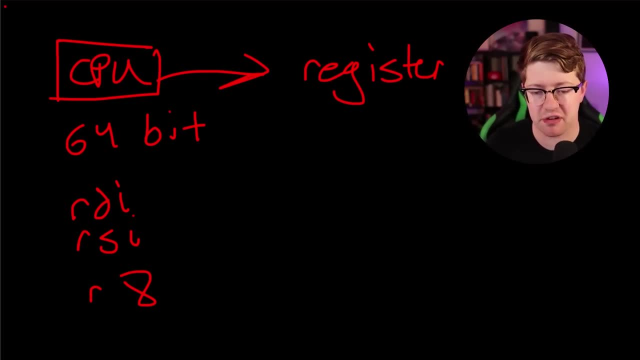 maybe R eight, for example. all of these are 64 bit registers And this are here. I think of it meaning really big, meaning that it's a 64 bit register. And also, before you ask: yes, I did lose my voice this weekend And yes, I did shave my beard off this weekend, It's been a weekend full. 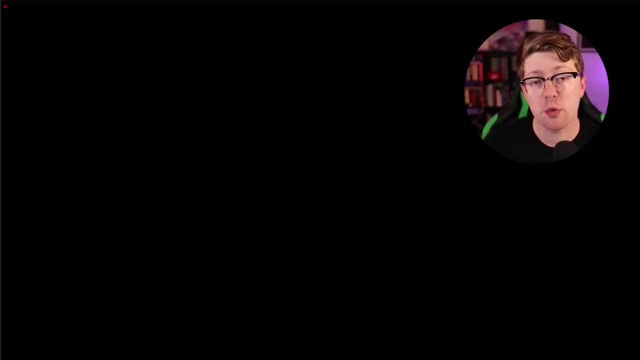 of events. Thank you for asking. So with these registers we can do a series of operations on them. We can move, for example, so we'll say, move RDI the number eight, that means, move the number eight, the constant value, into RDI. We can also move registers between each other, So we can. 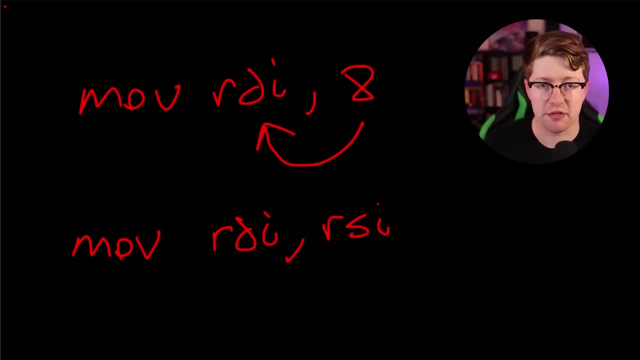 say, move into RDI the value in RSI. So these are both movements in and out of registers. Those are pretty simple. And then one of the more important ones we can do are called memory operations. we can move into RDI The value at- we call it the quad word pointer. 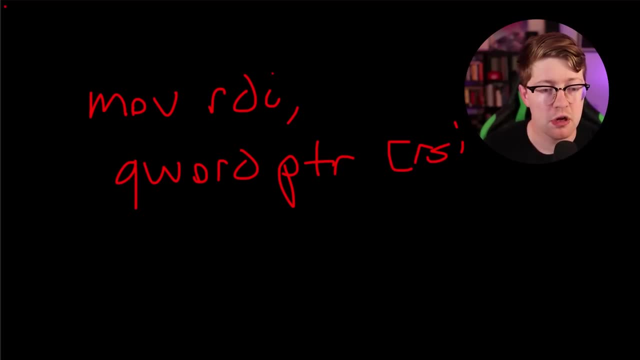 Of RSI, for example. what that means is it says: treat the value in RSI as a pointer and then remove the quad word length, that's eight bytes or 64 bits. remove eight bytes from memory and put it into RDI, And then we can do the opposite. we can do the same thing in reverse. we can say: move to. 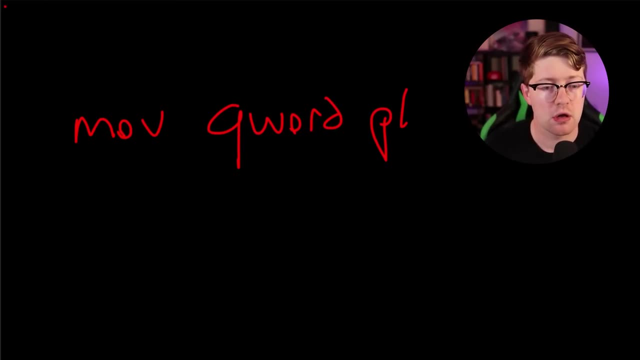 the quad word pointer in RSI, The value in RDI. So the first one was a load rate. we took values from memory and put them into registers. Now we can take values that are in registers and put them into memory. So this is a. 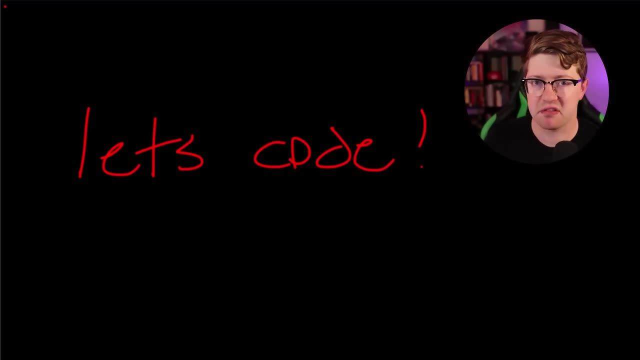 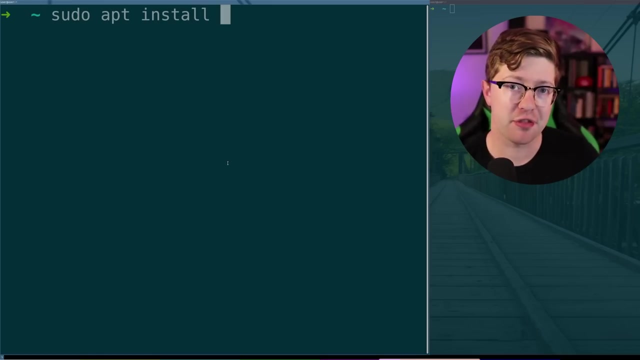 store operation. So, with the basics out of the way and again, if you're a little lost, it's okay. we're going to write some code now to kind of clear it all up. Let's get into our virtual machine and write some code. Okay, so to get started, we have to install the assembler and 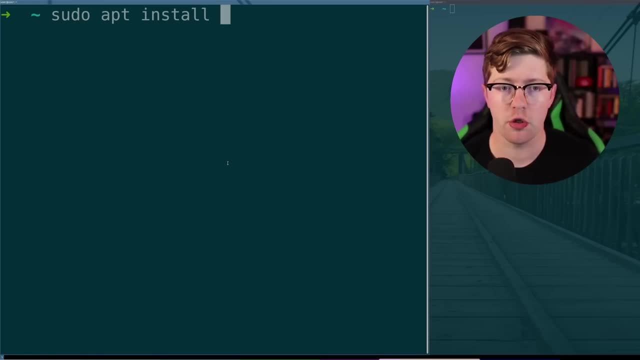 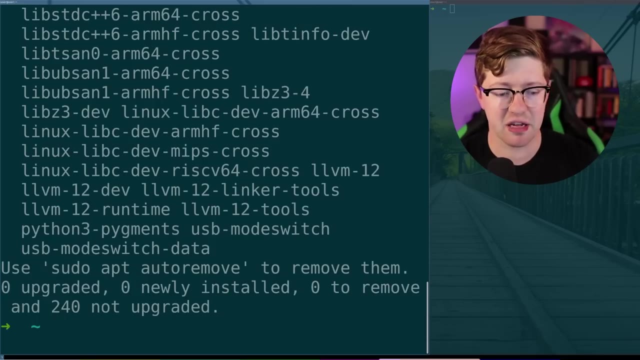 the linker that will allow us to compile our assembly code into machine code that runs on the computer. So to do that we have to run a sudo apt install gcc by running the assembly code. So running this will actually get the assembler as and the loader LD. I already have it so 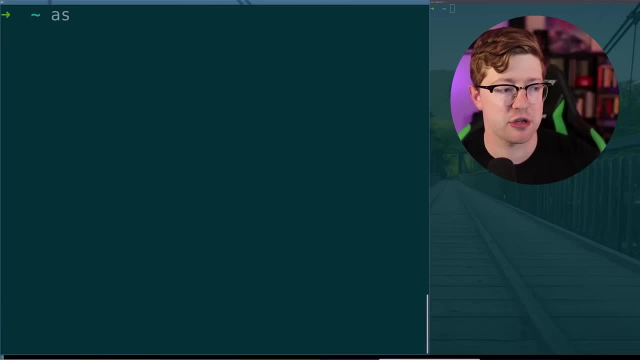 nothing happened here, But just to test that you have it. if you type as assembler, that should hang, meaning it's looking for an input file to assemble, So we're good there. And also LD, it should say no input files. if you have both of those that run, you should. 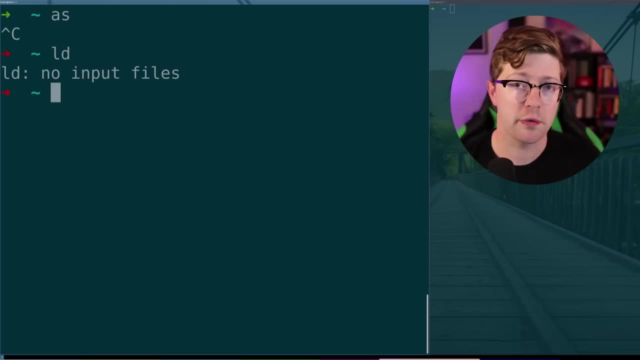 be able to follow along as well. So now let's actually write some code that we're going to assemble in our program. So in my folder, assembly tutorial, what we're going to do is we're going to open up our file. we're gonna say vim, sem dot s. you can name this. 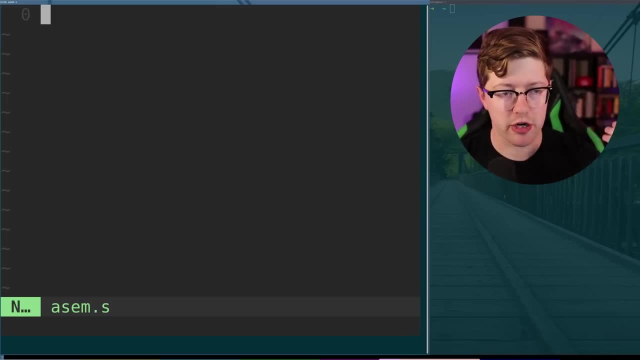 file whatever you want. And here we are. we're in a file that we're going to actually write our machine code, And before we write our machine code we have to start the file off with some boilerplate code that tells the assembler what to do. 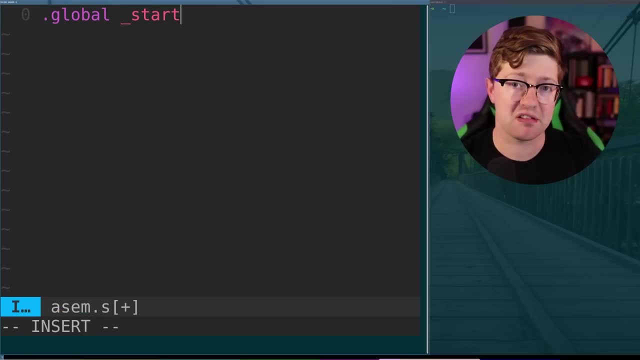 So the first one is global start. that exposes a symbol called start to the linker, so it knows where our code starts. And also we're going to say Intel syntax, no prefix. That makes our code a little easier to read and write for an average human being. So then, 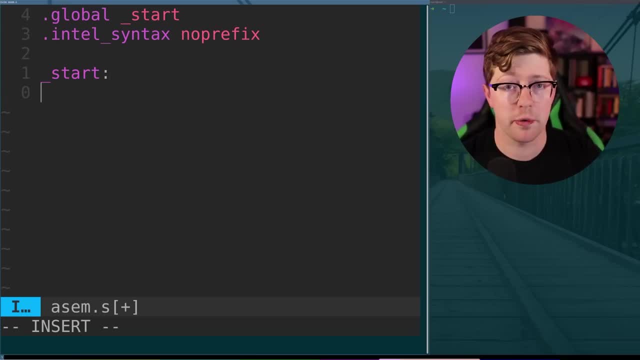 we can say: underscore, start and then a colon, and that is where our code is going to start. So if we write this and we get out of here, we're now going to try to assemble our code using the assemblers. we'll say as: 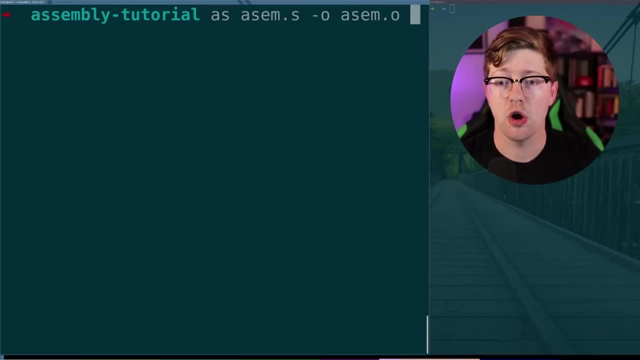 on our codes. we're going to say a semo, And there we go. So now we have a file called a semo. Now we need to invoke the linker to actually convert that into an executable elf, because right now this is an intermediate object. we can't actually run this. we have 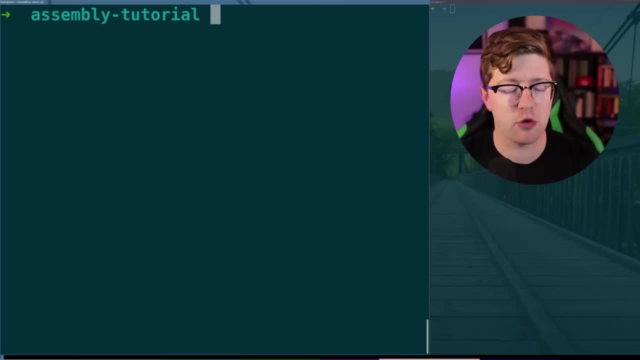 to use the linker to make it a full elf that runs. we can use the linker itself or we can use GCC. we're gonna use GCC and say GCC, tack, oh, a sem, do that on a semo. we're. 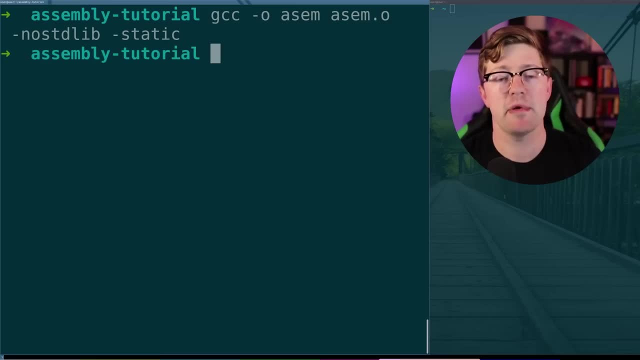 gonna say no standard lib and tack static. that makes it so that the binary doesn't get any additional stuff in there from lib C and makes it easier to run. So if we run this file we are going to get a crash And there's a reason for that. we haven't told the binary. 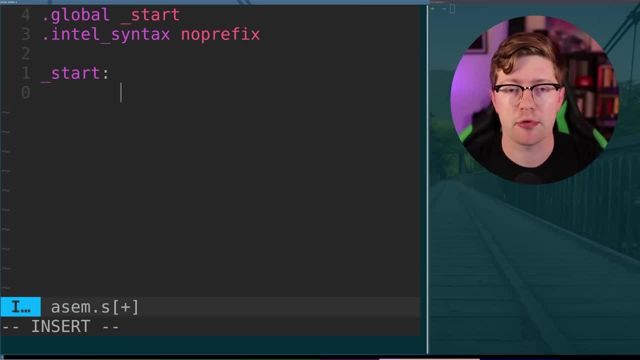 how to properly exit. So we can go back into our file here And we can do some operations that we talked about in our previous example, when I was talking about the registers. right, we can say things like move RDI, the number eight, and we can say move into RSI, the value. 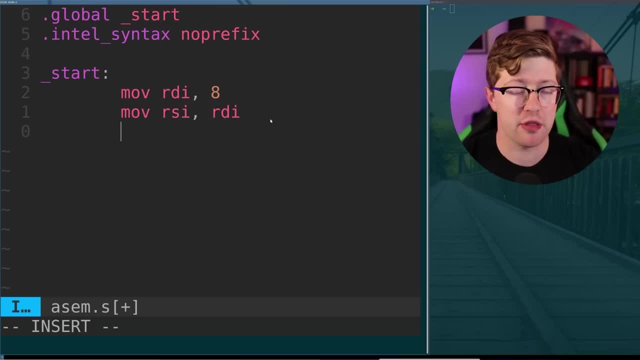 of RDI And at the end of this code, both RDI and RSI- the registers will have the value eight in them. So that's pretty cool. Let's go back and rerun our command. So again, we use AS. 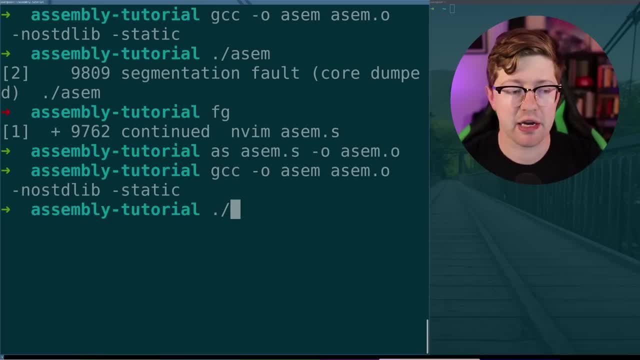 to assemble it. we use GCC to compile it And then we can use that and run the programs And you're going to see we get a crash again. So those operations actually did happen under the hood. when it got to the end of our code, it didn't know how to exit our program. you. 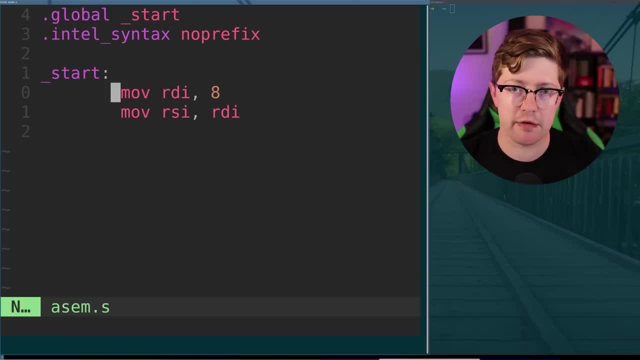 may be asking. you know we have these operations to move values in and out of registers, in and out of memory. But how do we make the computer do something? How do we make it print data or properly exit our process or do something that matters? 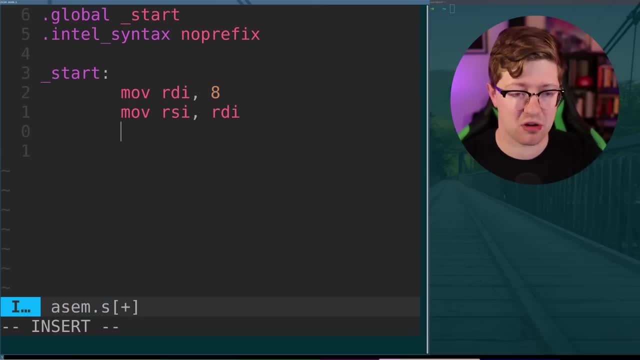 to us as human beings. To do that we have to invoke what is called a syscall, And the actual instruction and assembly to do that is called a syscall. Now it's a little more complicated than just typing the word syscall. we have to set up the registers in a particular 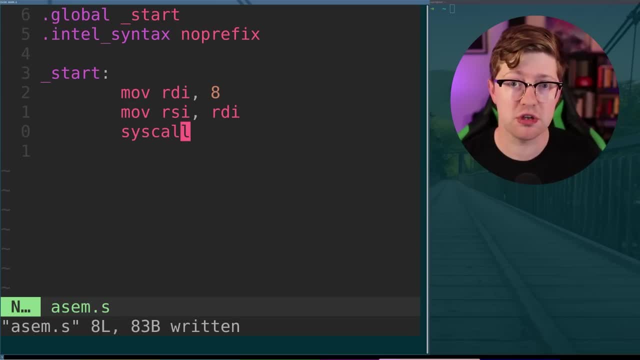 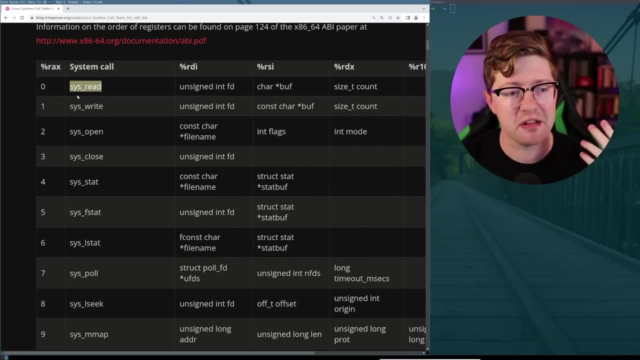 way that the kernel beneath us understands what to do. what is the question that we're asking the kernel to do for us? So what I'm looking at here is what is called a syscall table. This is a list of all the operations the kernel 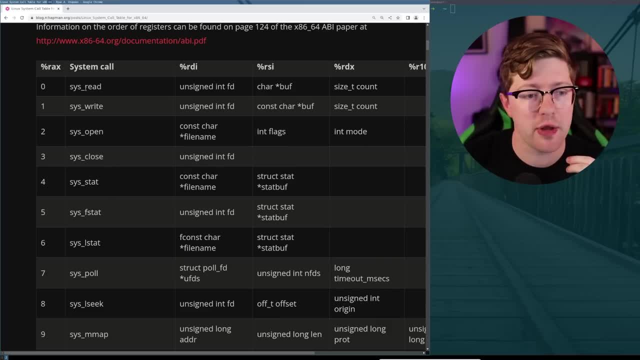 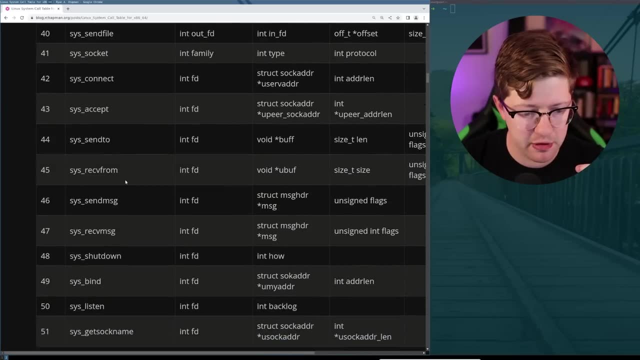 is able to do for us. when we invoke a syscall- And as you can see here we have things like sys. read sys right, we have sys exit in here somewhere. let's see if we can find it. I'm pretty sure it's like syscall 62, or something 60,. there we go. So you'll see that we have. 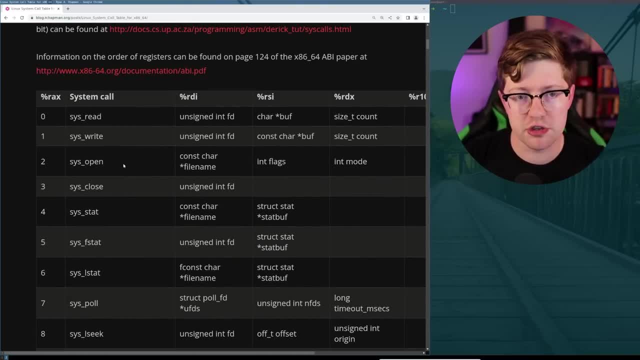 all these things we can ask the kernel to do for us. The way we ask the kernel to do them is: before we invoke the syscall, we have to set up the registers in a way that the kernel recognizes our command. So here we have register rax. that means, for example: 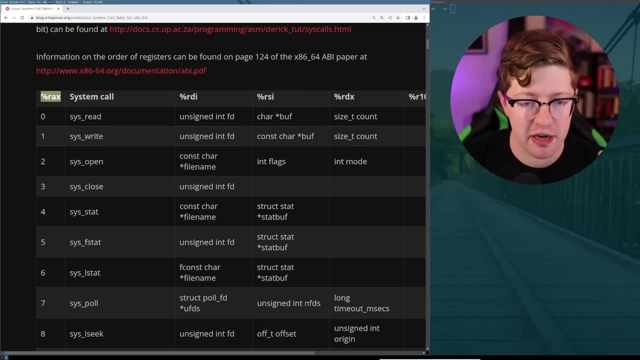 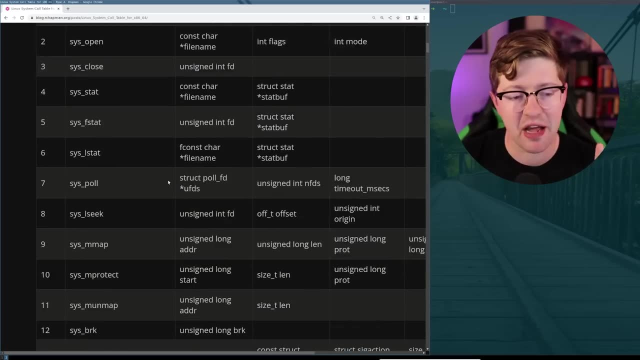 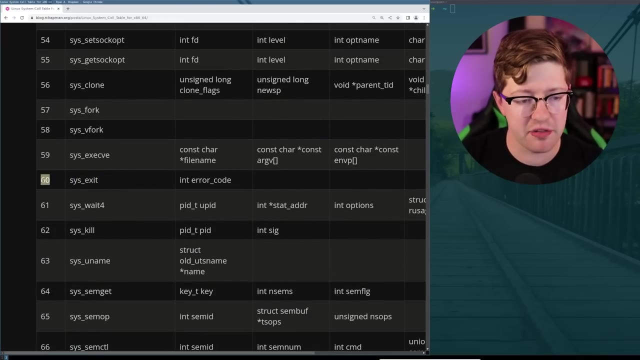 to do the sys read operation. we want to put the zero into the rax register. we also put the file descriptor number. we want to read the buffer we want to read into, etc. So let's test this out With the exit syscall again, it's going to be syscall number 60 here. So we put into rax the number 60. 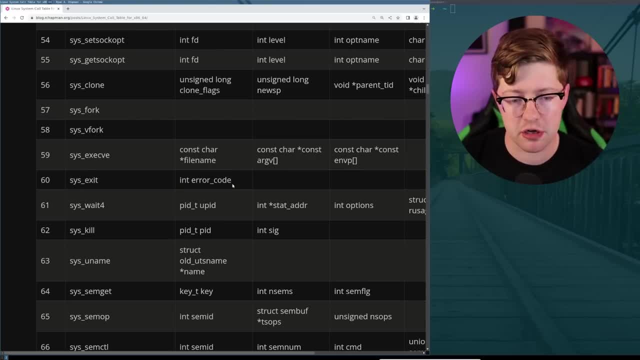 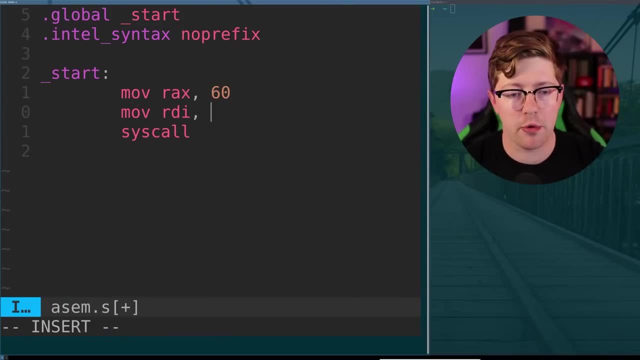 And then into RDI we put the error code we want our process to return with. So let's, let's try this out. So we say we wanted to put the number 60 into rax and then into RDI. we wanted the error code, And I'll show you how to check that at the end of this run. 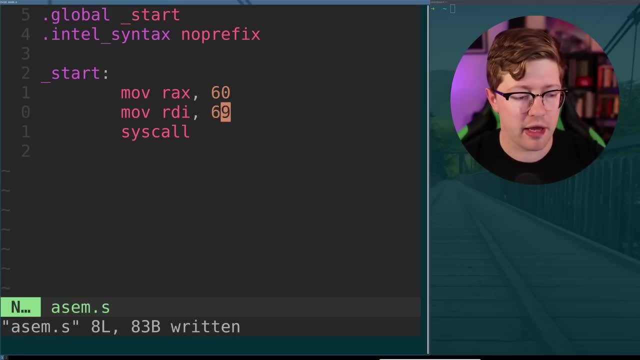 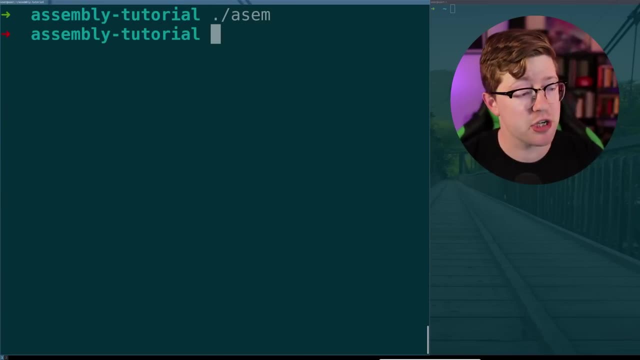 We're gonna try the number 69 real quick. So let's do that, And we're going to reassemble our program, we're gonna run GCC on it And then if we run our code, our program didn't crash. And the reason for that is we told it how to exit, we gave it the instruction. 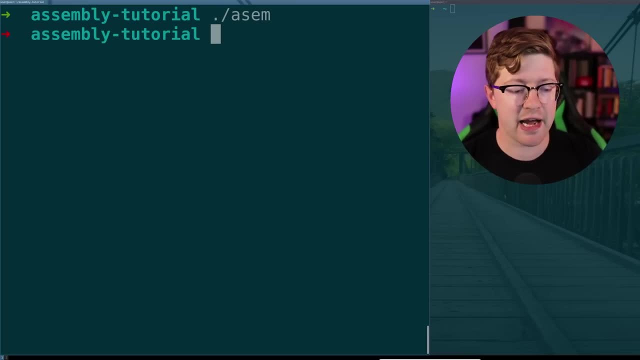 from the kernel to exit. And now we're gonna check the exit code to see if it's actually doing what we asked it to do or something else. So we'll do echo $ And boom, the return code is 69, which means that this is the code that we ran. So let's level this up. Let's. 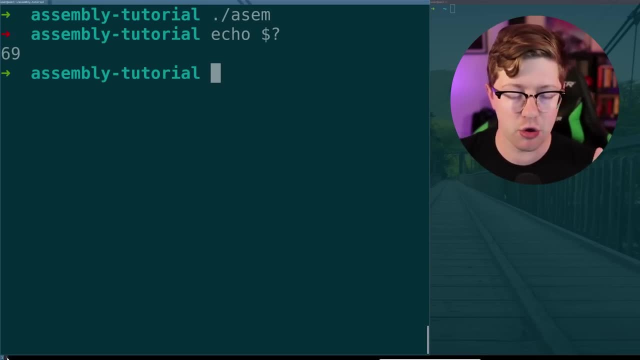 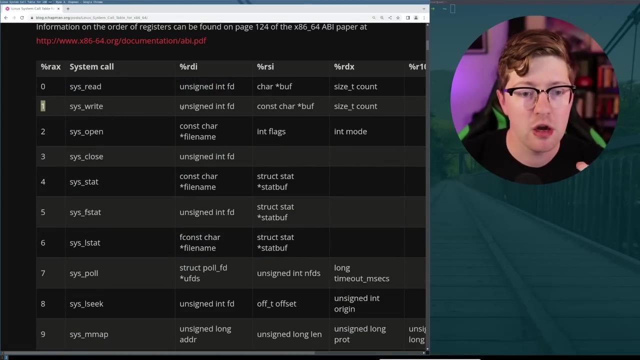 add another layer to this. let's make the program print a string: Hello world. the way we did the Hello world operation is: we're going to invoke a syscall called sis. right, we're going to put one into rx To do that. we're going to write out to the standard out. 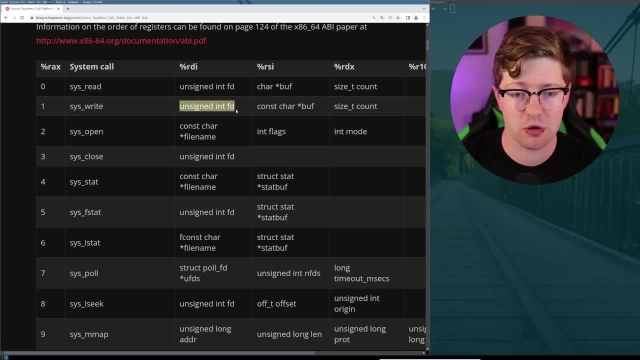 file descriptor, which is file descriptor number one, in out an error 012.. And we're going to write out a buffer that contains our Hello world string And also we're going to put into rdx the number of bytes to write. So let's add that into our program real quick. 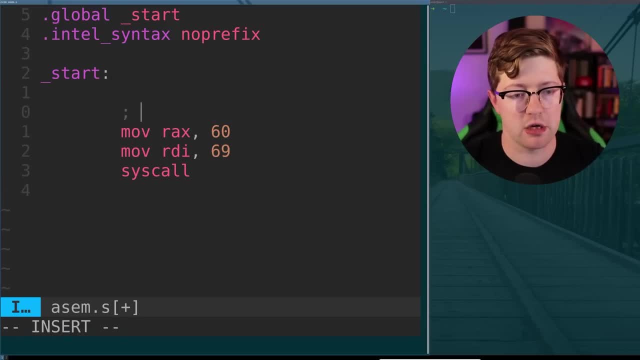 So we're going to leave this in here, because this is actually just us exiting. So we'll add a little comment here. we'll say: this is the sys exit call, And then we're gonna do the sys write call. To do the sys write sys call, we have to do a few things Again. 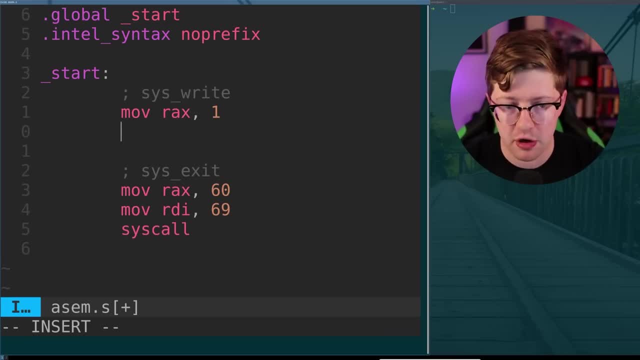 first we have to tell rx what sys call we're doing. So we move one into rx. we need to put the file descriptor into rdi. So remember, standard out is file descriptor number one, So we'll also put one here. then we're going to move into our si the address of the buffer. 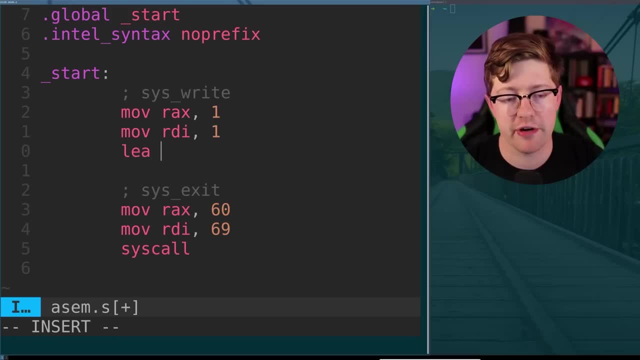 that contains our string. So this is actually going to be a new operation called load effective address, And then we're going to define that here in a second. And then, finally, we move into rdx the length of our buffer, which is just going to be 13,. we can hard to code that into. 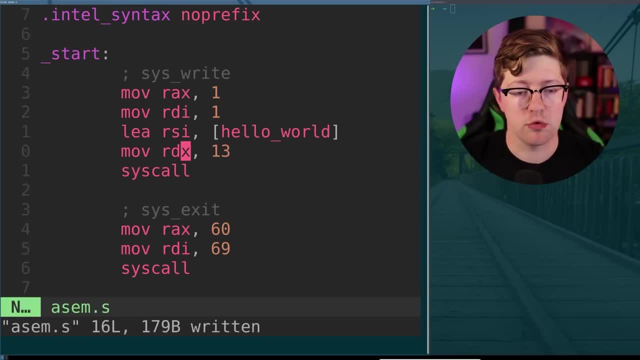 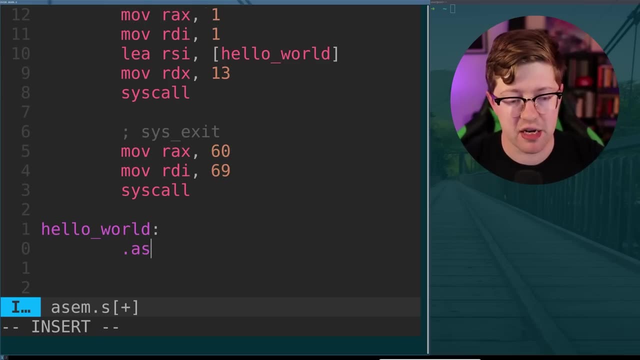 our code right there And then we'll invoke the sys call And then we'll go from there. Now we can do down here is we can create a new symbol called Hello world with a colon, And we're going to say: it's an ASCII string, zero, delimited. that'll be Hello world exclamation. 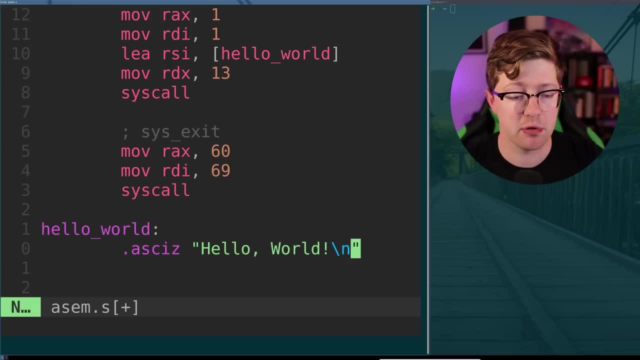 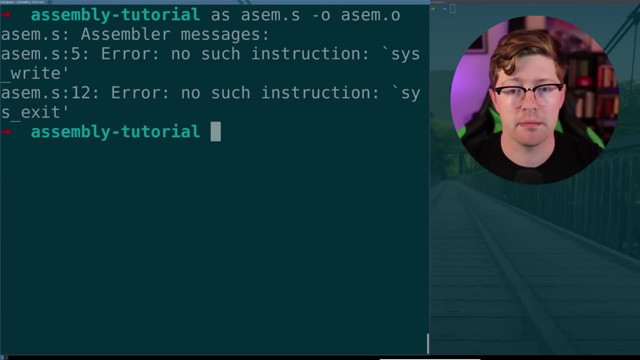 point, new line, and then a zero will come at the end of that like a colon. So we're going to call it. ASCII is supposed to have. So we can do that, we can save it, we can quit, And now we'll do the same thing as before. we can type as to assemble our program. Oh,